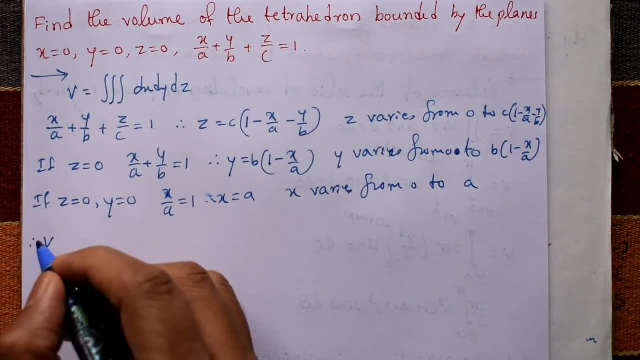 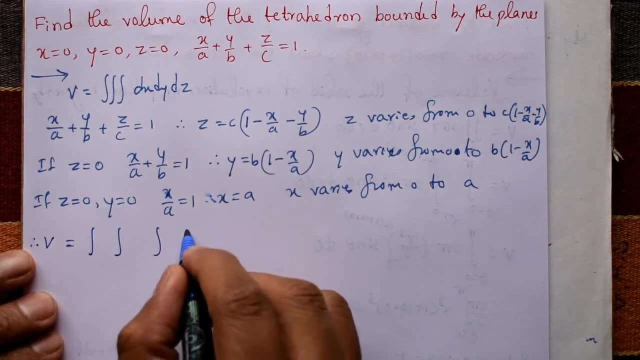 Now therefore, v is value that is equal to integration, of integration, of integration, integration- This is the solution. Okay, that is why I am agreeing with Tambrapath again- is first, I'll take dz, d by dx. first, integration is with respect to x. this one, that is x, is equal. 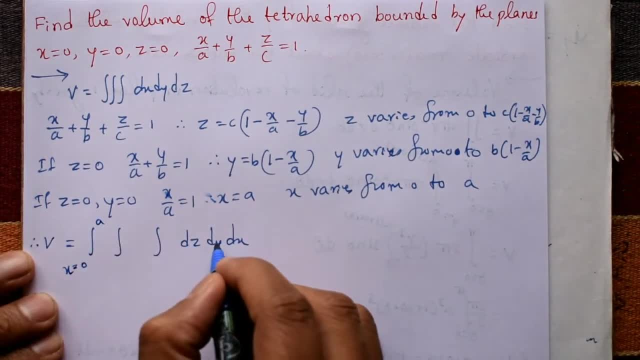 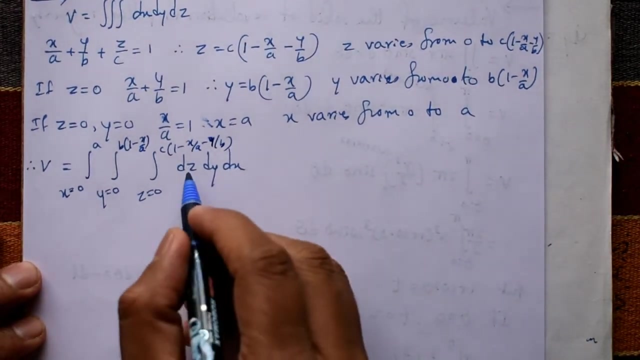 to 0 to a, x. where is form? second one is: means this one with respect to y. second integral: y is equal to 0 to b into 1 minus x by a. and the third one means, with respect to z: z is equal to 0 to c into 1 minus x by a minus y by b. okay, integrate one by one. first with respect to z: 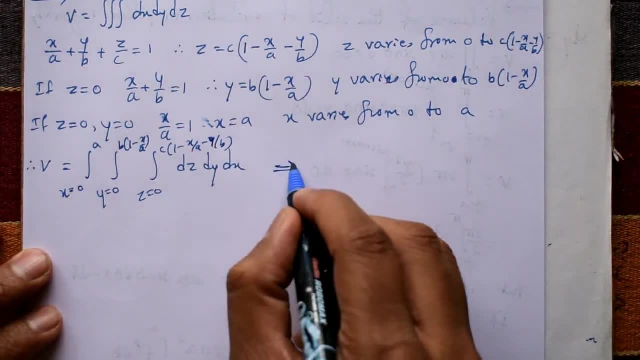 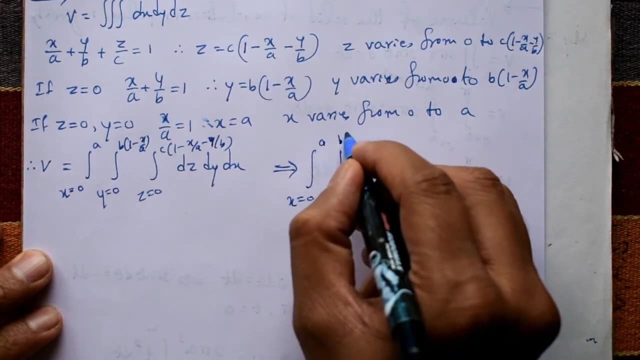 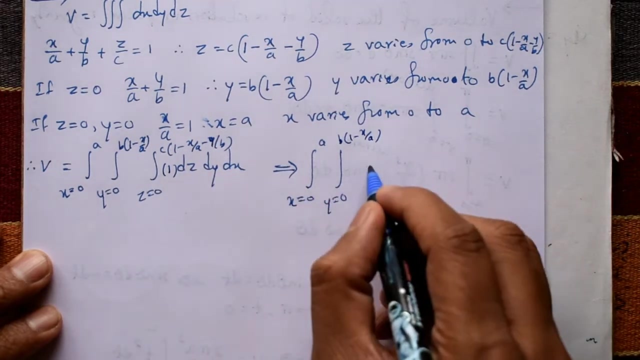 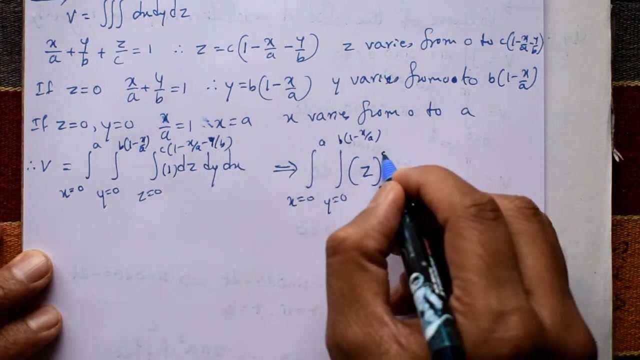 and this is equal to integration of x is 0 to a, integration of y is a. 0 to b into 1 minus x by a. now, integrate with respect to z- one is there- with respect to z- means z integration, one with the spirit: z is a, z only, and 0 to c into 1 minus x by a, minus y by b. and 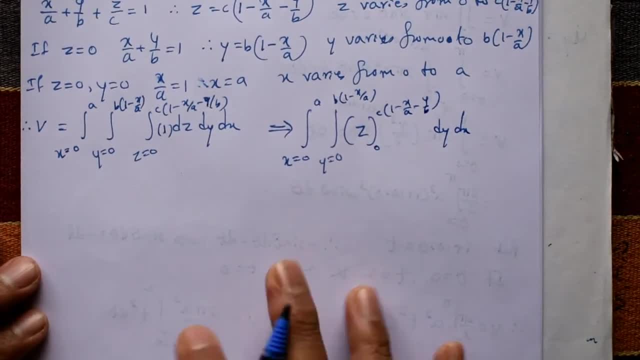 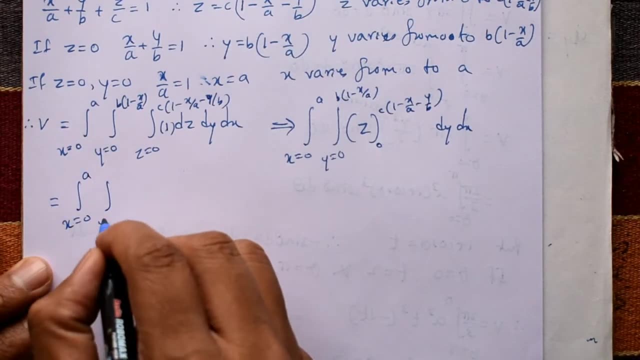 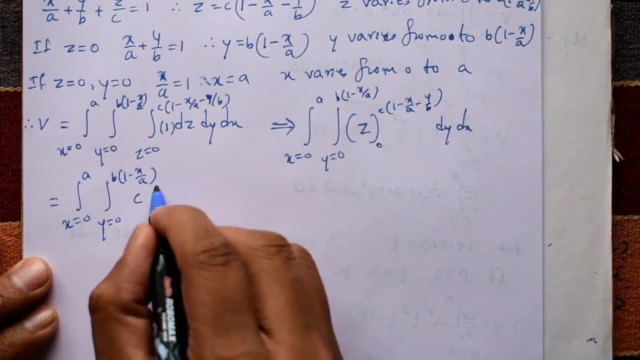 with respect to y with respect to x, as it is okay now, this is equal to: integration of x is 0 to a. integration of y is 0 to b into 1 minus x. by a. take upper limit z is equal to upper limit c into 1 minus x. by a minus y. by b minus lower. 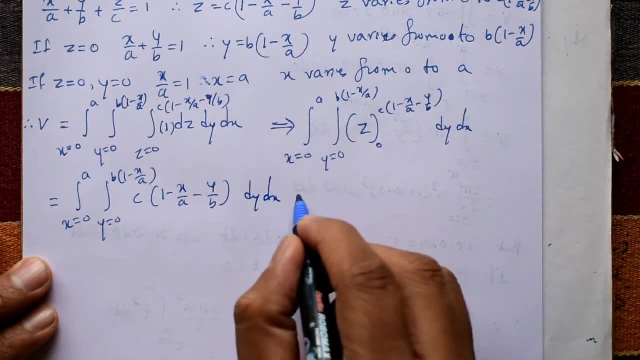 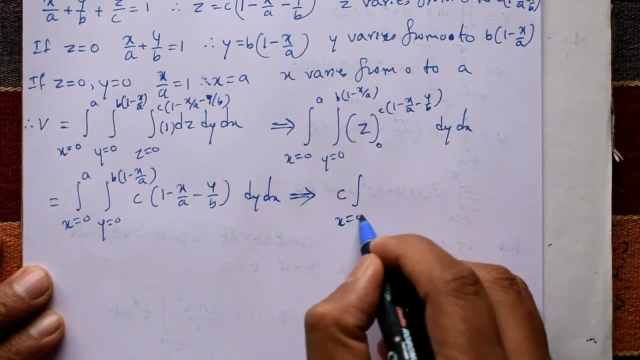 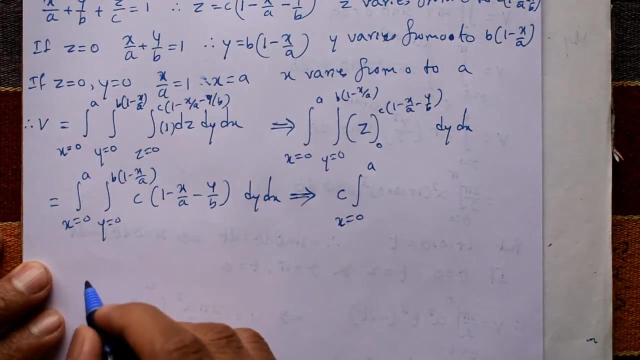 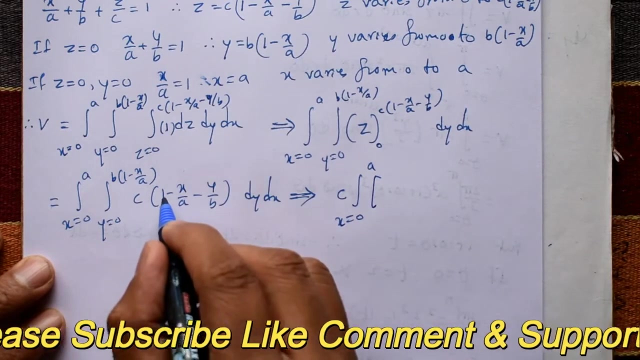 0 means 0 only. now, dy, dx, okay, this is equal to c, is a constant. take outside c. integration of x is 0 to a. now integrate with respect to y, these three terms. with respect to y, only x, a, b treated as a constant. okay. now integration of 1 with respect to y, is a, y only minus x by a constant, again it. 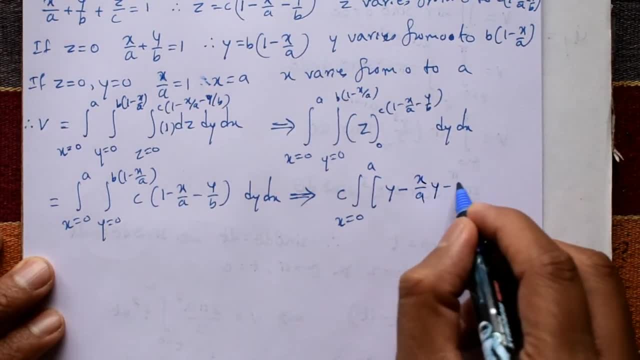 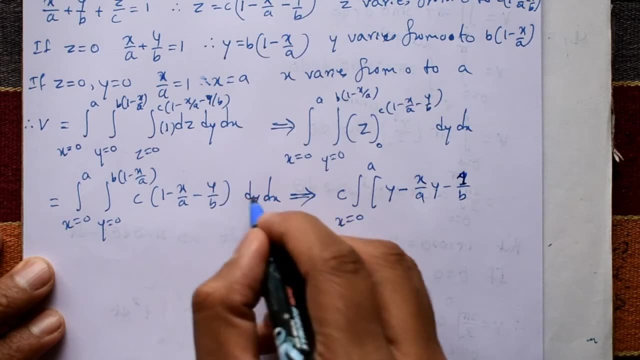 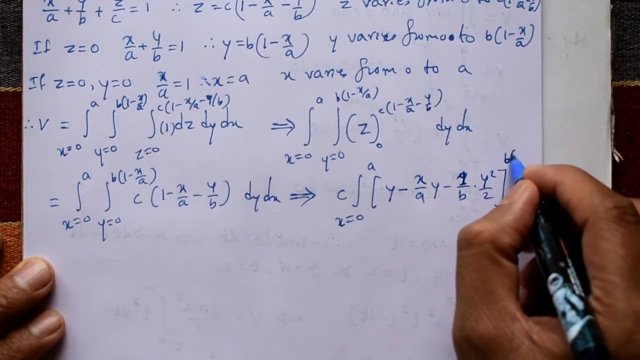 is 1 with respect to y, that is y only minus y by b. sorry, 1 by b, sorry, it is 1 by b. and integration of y with respect to y, that is a y square by 2, and limit 0 to b into 1 minus x by a and with: 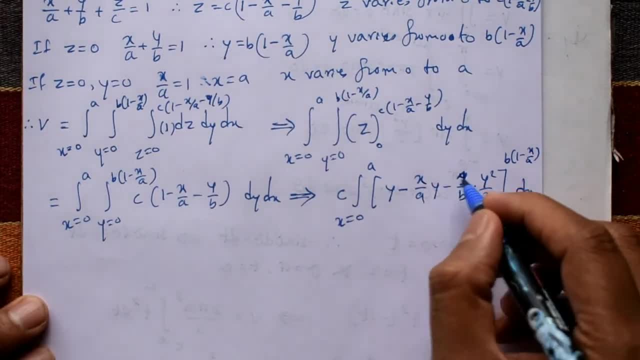 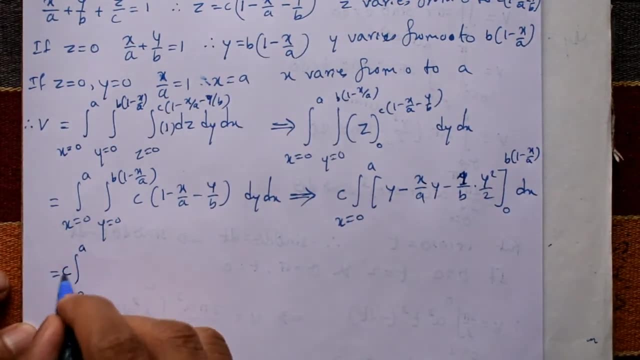 respect to x as it is. now. take upper limit minus lower limit and this is equal to x, is 0 to a plus. this is outside. now take y is equal to upper limit, y is equal to upper limit, that is a b into 1 minus x by a minus lower limit. 0 means 0, only minus x by a second term. take upper limit. 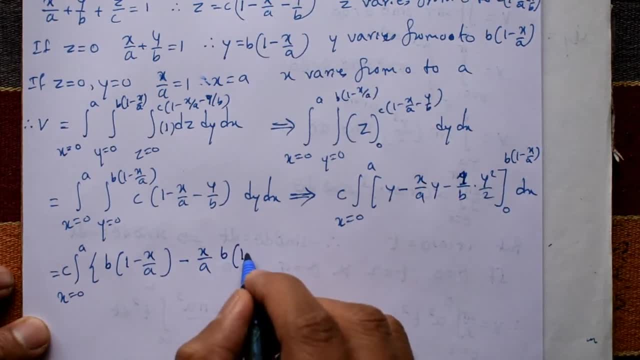 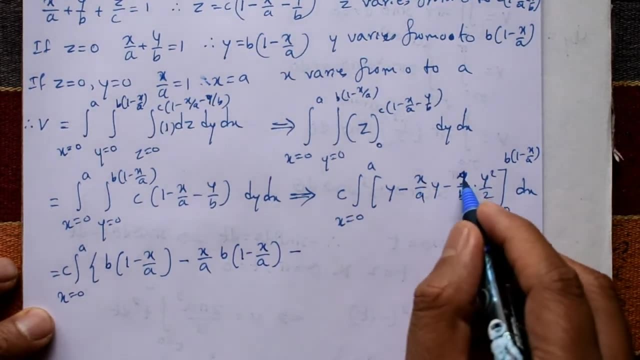 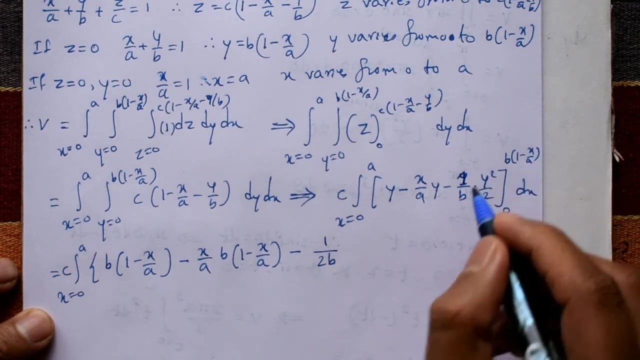 y is equal to that is a b into 1 minus x. by a minus y is equal to 0, means 0, only minus. okay, 1 upon 2b, 1 by 2b, 1 upon 2b. take y is equal to upper limit y square. only that is a b square. 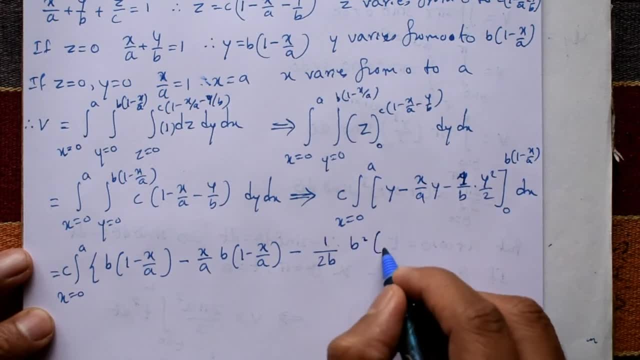 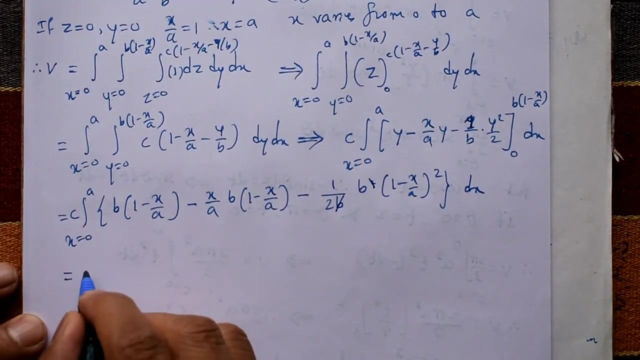 into 1 minus x by a whole square, because this is a y square. now, with respect to x minus lower limit, 0 means 0, only 1, b is a. cancel this is equal to c into integration of x is a 0 to a. Now take b into 1 minus x by a b into 1 minus x by a, b into 1 minus x by a. take. 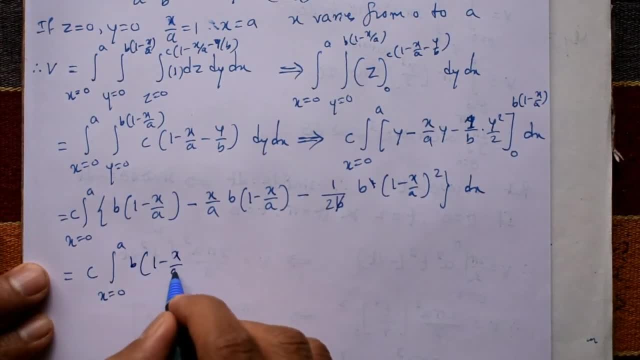 over 1, that is a b into 1 minus x by a. Now inside is this term is 1 minus x by a. remaining minus b by 2 is remaining okay, that is a b by 2.. And one more bracket: 1 minus sorry 1 b is taken outside sorry 1 by 2, and 1 bracket. 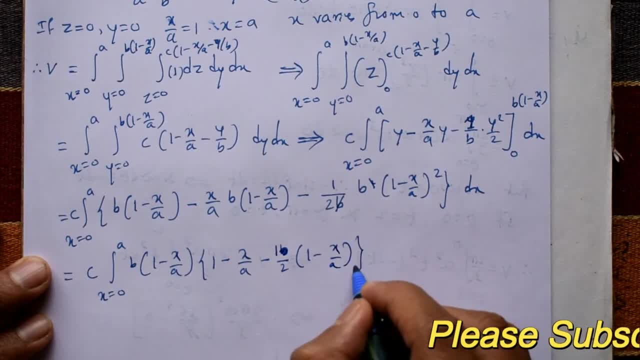 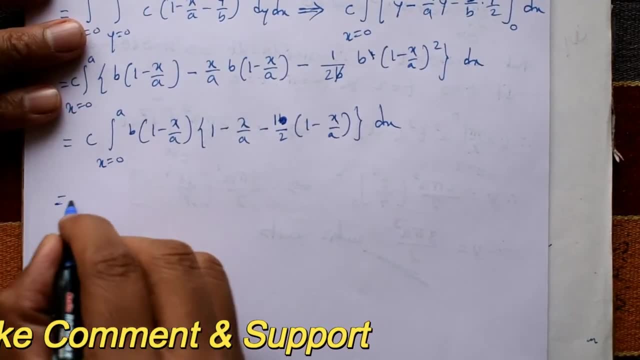 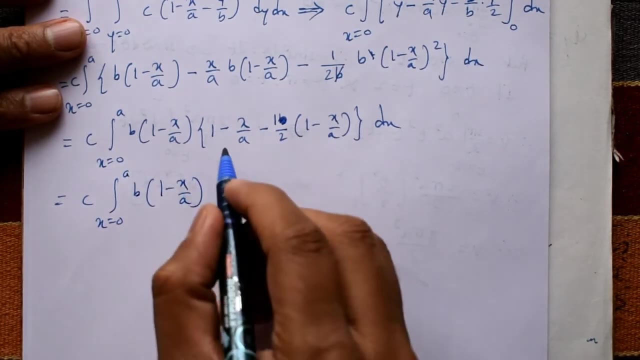 is remaining 1 minus x by a and with respect to x. okay, Now this is equal to c into integration of x is 0 to a, b into 1 minus x by a. open the bracket 1 into minus half. that is plus half plus half minus x by a, minus into minus plus.